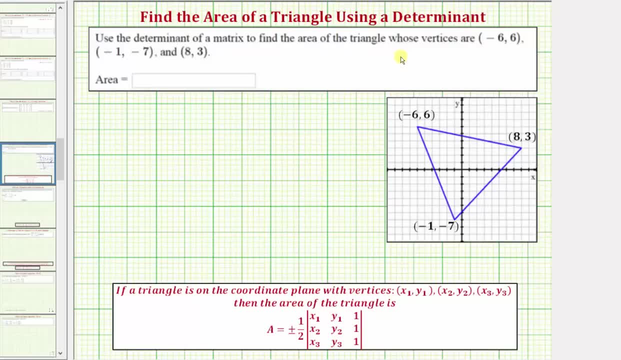 We want to use a determinant of a matrix to find the area of the triangle whose vertices are given here. Notice how I've also graphed the vertices, as well as the triangle, on the coordinate plane. If a triangle is on the coordinate plane with the vertices shown here, then the area of the triangle is equal to plus or minus. 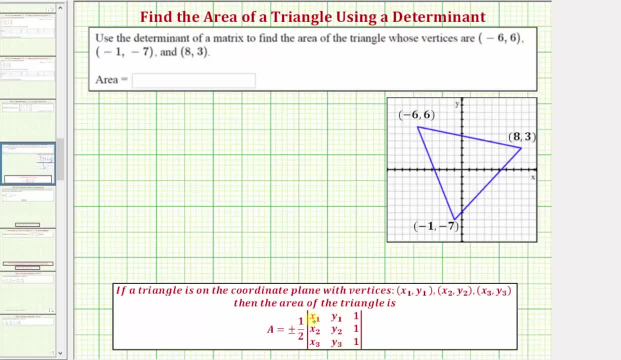 1 half times this 3 by 3 determinant, Where the first column of the determinant is equal to the x-coordinates of the vertices, the second column of the determinant is equal to the y-coordinates of the vertices and the third column is all ones And the reason there's a plus or 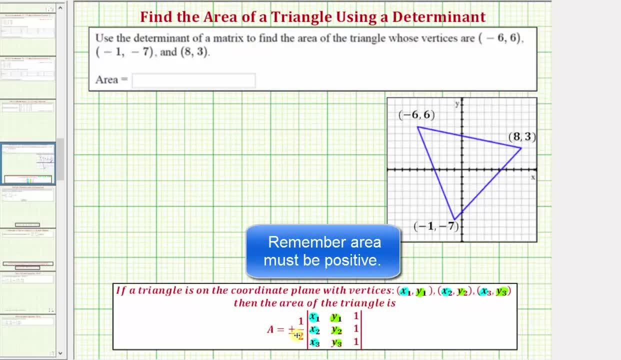 minus. here is: if the value of the determinant is negative, we'd have negative 1 half times the determinant, And if the value of the determinant is positive, we would use 1 half times the determinant. So let's go ahead and set this up. The area is equal to plus or minus 1 half. 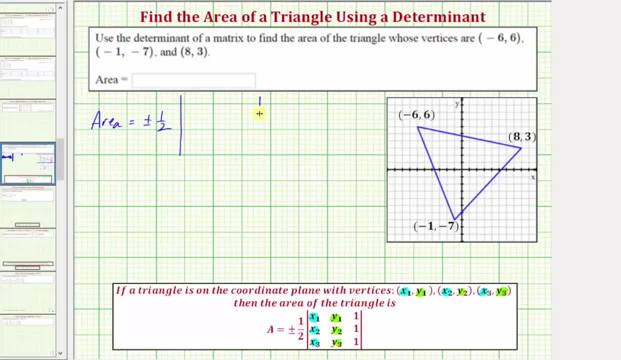 times the 3 by 3 determinant, where the first column is going to be negative 6, negative 1, 8.. The second column is going to be 6, negative 7, 3.. The and the third column will be all ones. 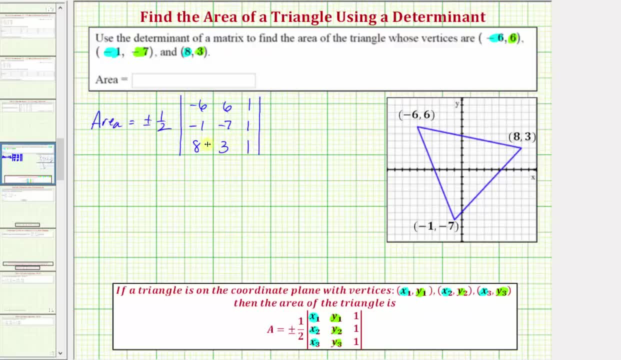 And now to evaluate the three by three determinant, let's go ahead and use the expansion by minors or the cofactor method, So we'll have the area equals plus or minus 1 1⁄2, and let's go ahead and use this first row here. 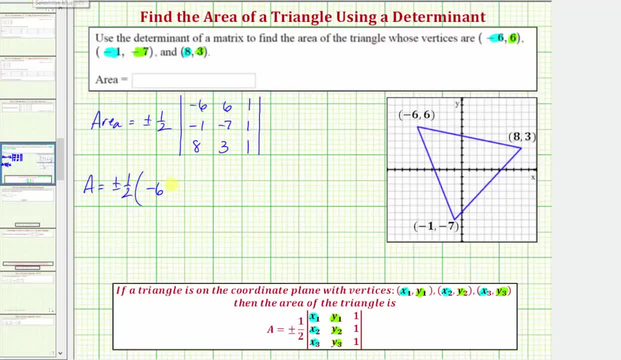 So we'd have negative six times the minor, which will be a two by two determinant that we form by eliminating or deleting the row and column of negative six. so we eliminate row one, column one, So we have negative seven: one, three, one. 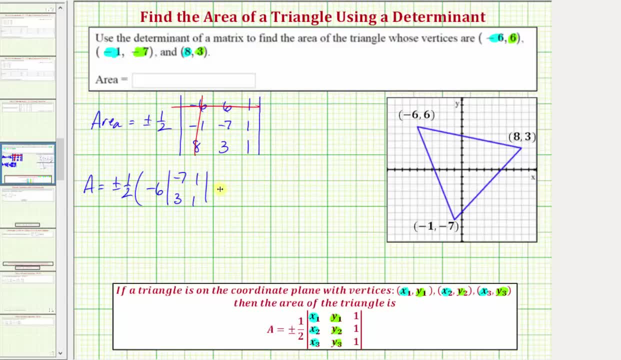 Now remember: if we're using the first row, we're going to have minus, and the next element in row one is positive six. so we have minus, positive six and then we have the minor, which is the two by two determinant formed by eliminating the row and column of this element.